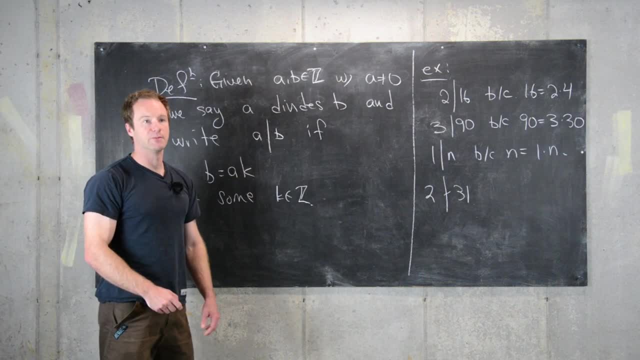 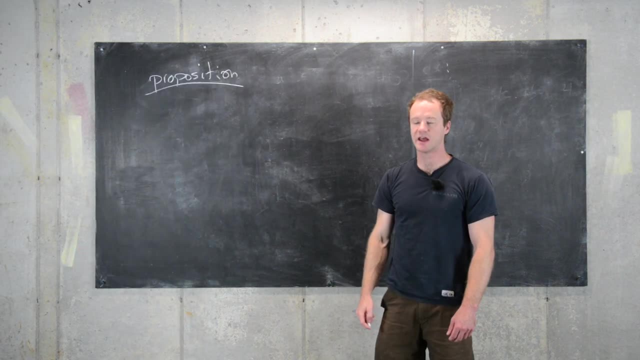 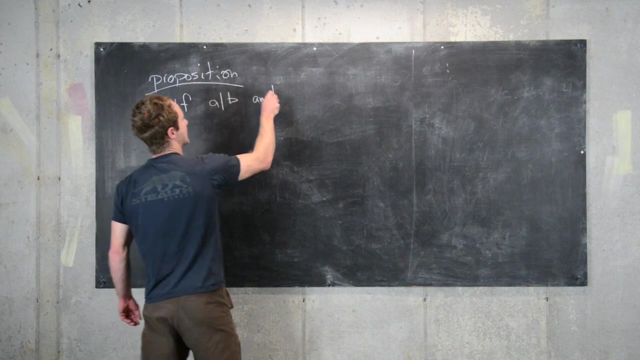 I want to clean up the board and then give an important result involving divisibility. Okay, here we want to look at an important result involving divisibility, So it'll have 3 parts. So the first part is as follows: If A divides B and B divides C, then A divides C. So there's some notion of transitivity among divisibility. Okay, great. So the next one is: if A divides B, then C times A divides C. 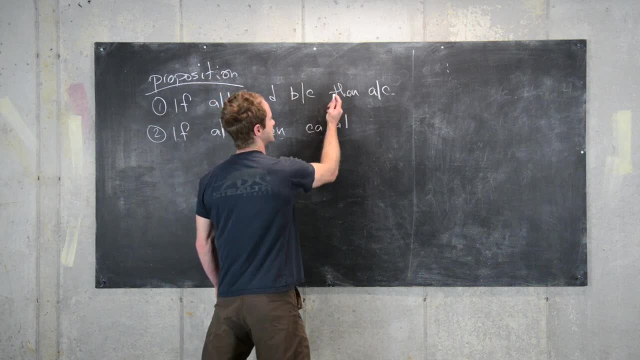 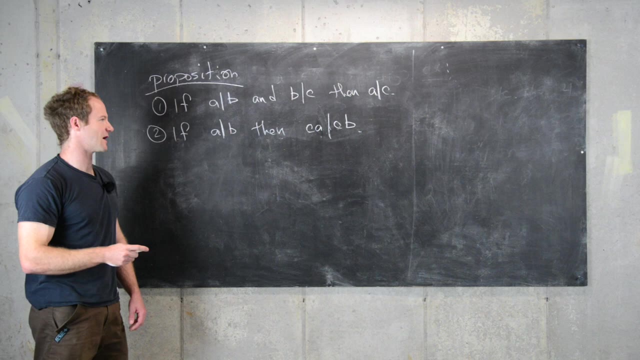 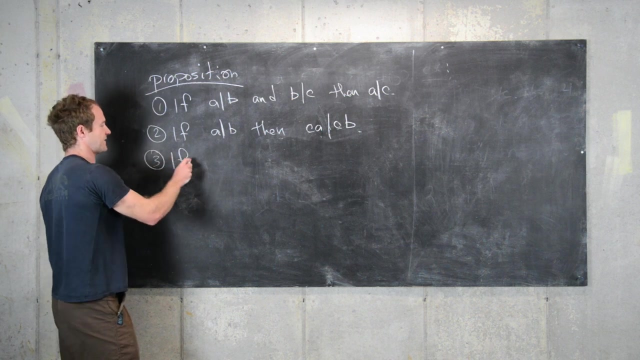 A divides C times B: Great. So obviously I'm leaving off some slight hypotheses about these numbers, A, B and C, But it's easy to fill in those details. And then, lastly, is if A divides B and A divides C? 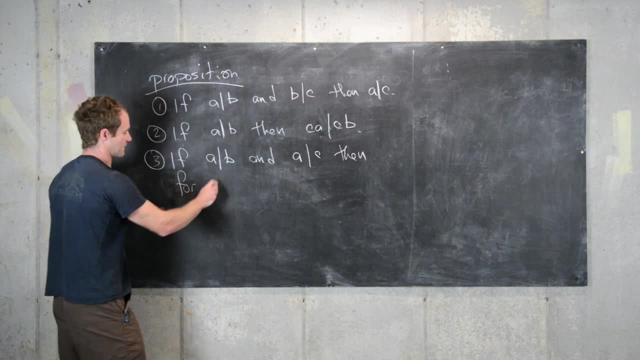 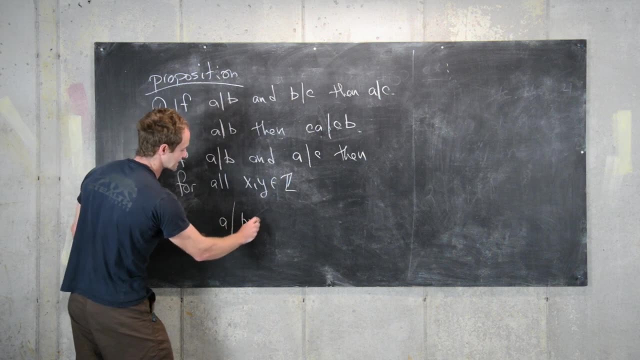 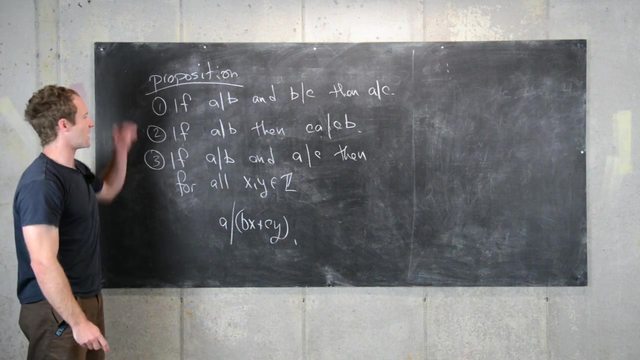 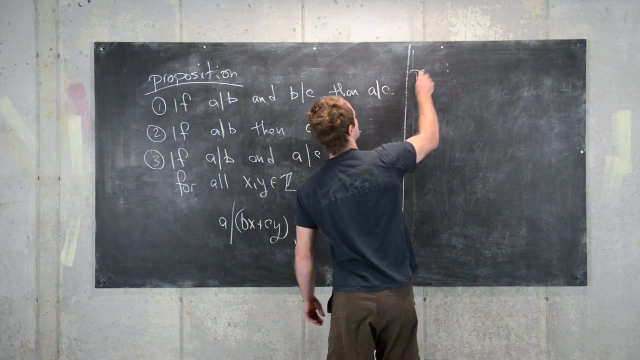 then for all integers X and Y, we have A divides BX plus CY. Good, So I don't want to prove all of these. Maybe I'll prove number one and then the last two will be left as an exercise. So proof for number one. 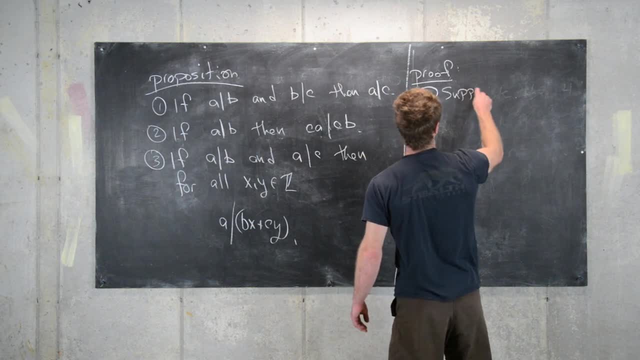 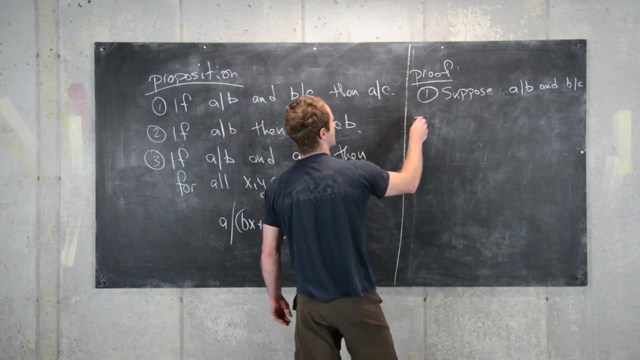 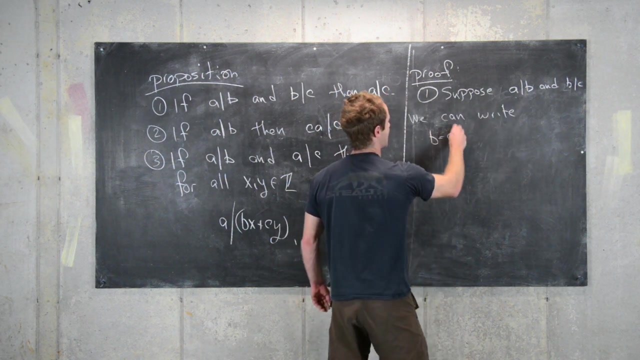 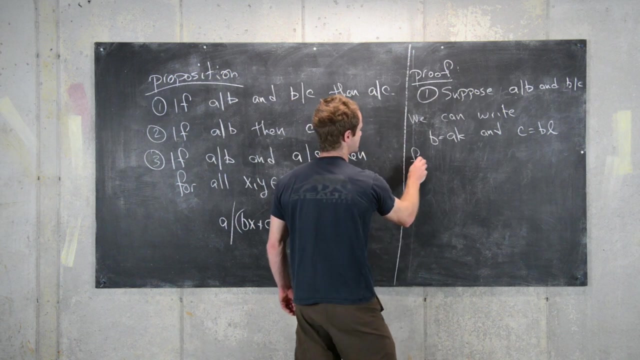 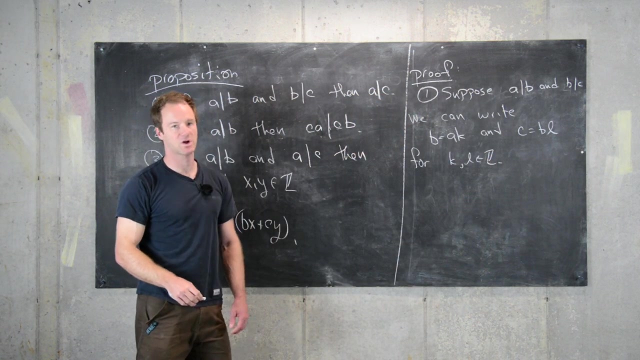 So let's suppose that A divides B and B divides C. So that means we can write: B equals A times K and C equals B times L for K and L some appropriate integer Good. The next thing we do is we match these two equations together. 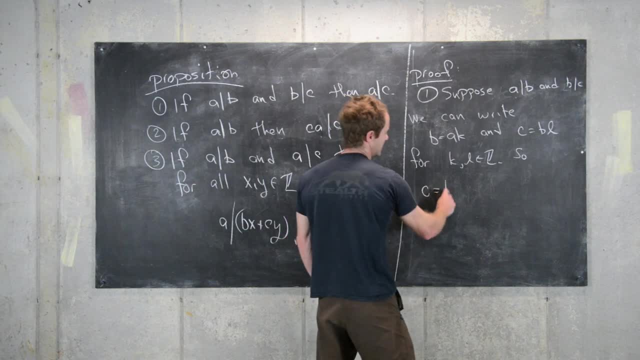 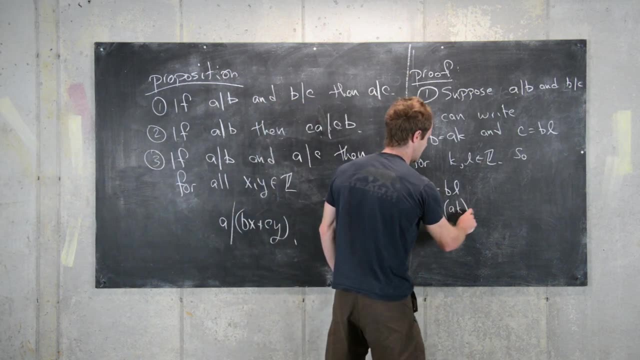 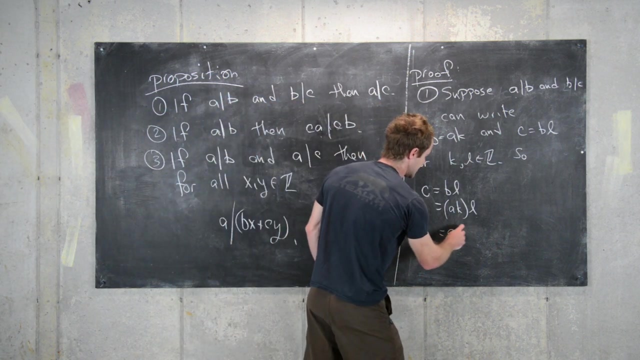 And that will give us C equals B times L, which equals- we'll replace B with this, So that's A times K times L. Good, Now we can re-associate, So that gives us A times K times L, which is A times K prime. 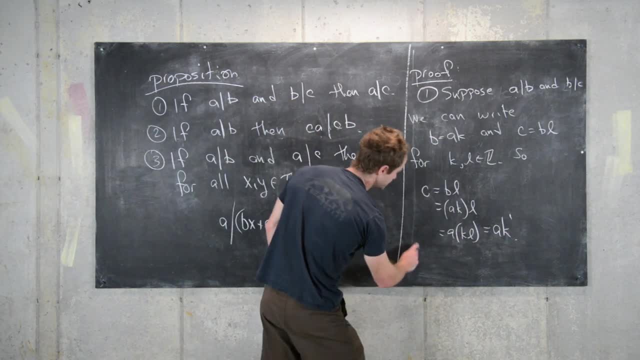 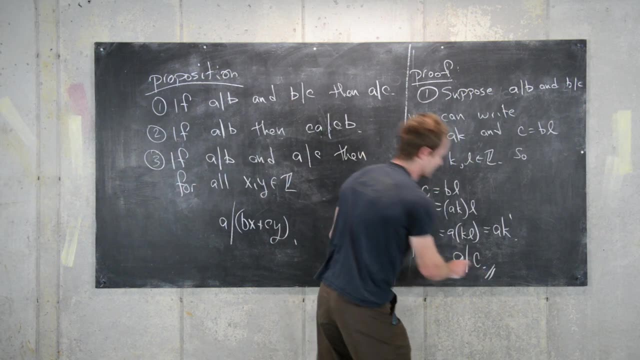 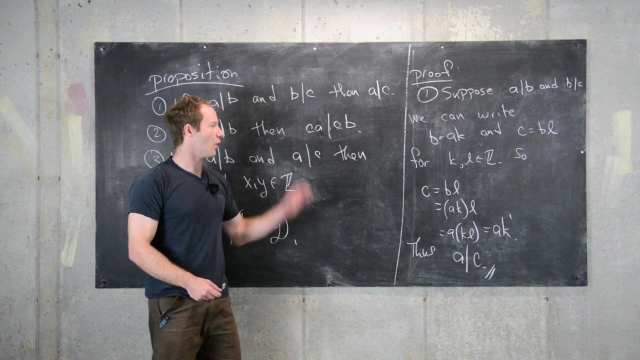 And K prime is A times K prime, And K prime is A times K prime And K prime is another integer. Thus we have A divides C, as desired. Okay, good. So before we end this video, I want to give one more result about divisibility. 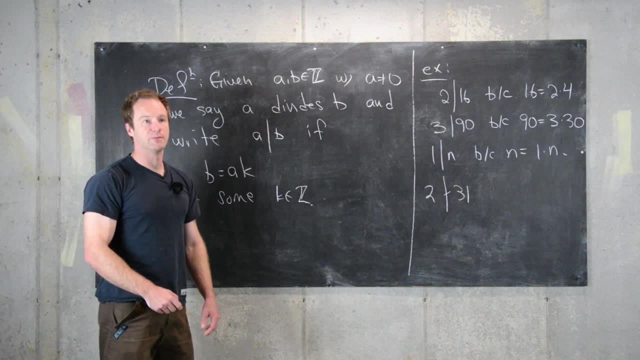 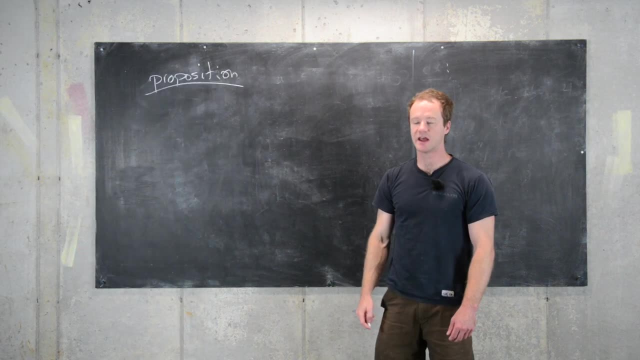 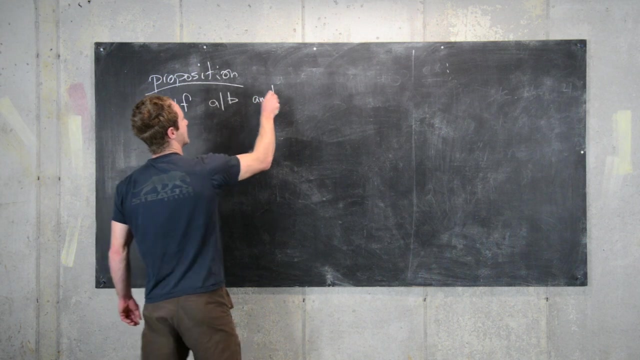 I want to clean up the board and then give an important result involving divisibility. Okay, here we want to look at an important result. It'll have 3 parts, So the first part is as follows: If A divides B and B divides C, then A divides C. 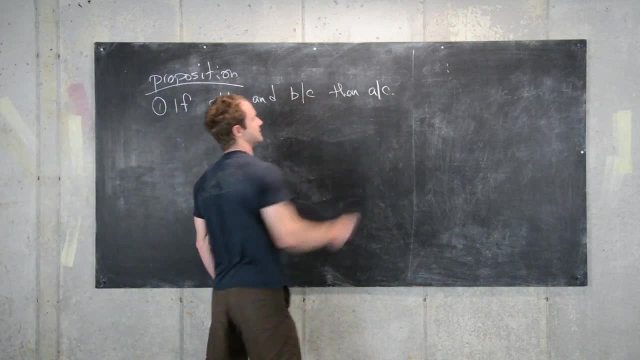 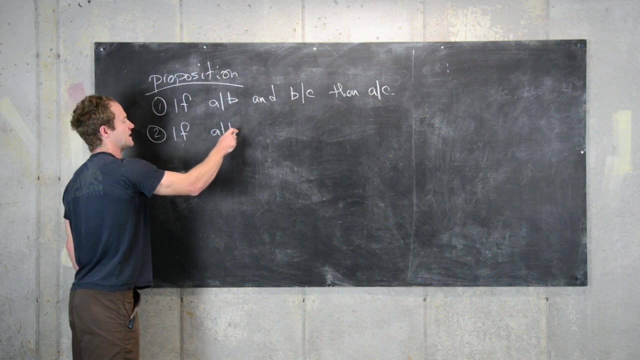 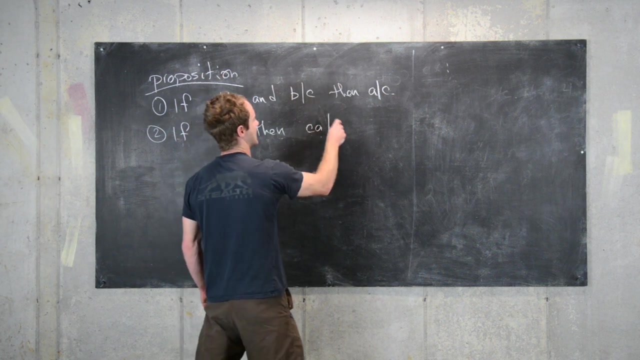 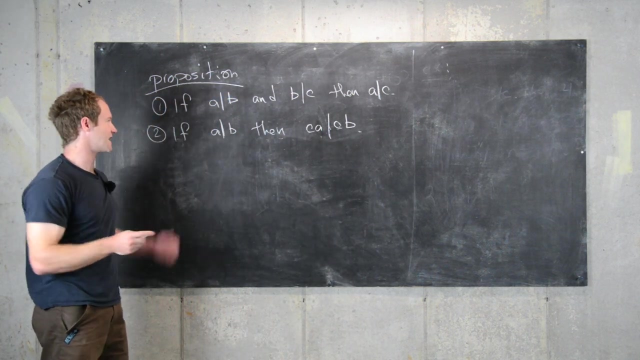 So there's some notion of transitivity among divisibility. Okay, great. So the next one is: if A divides B, then C times A divides C. A divides C times B- Great. So obviously I'm leaving off some slight hypotheses about these numbers: A, B and C. 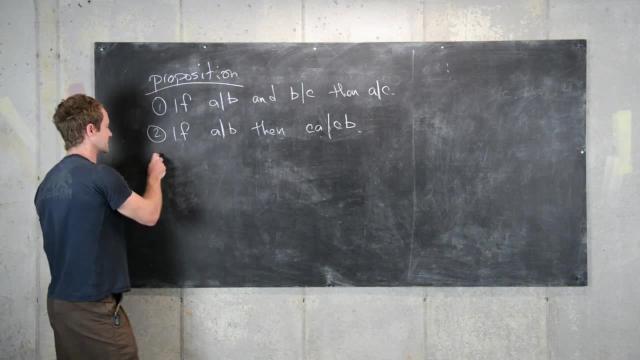 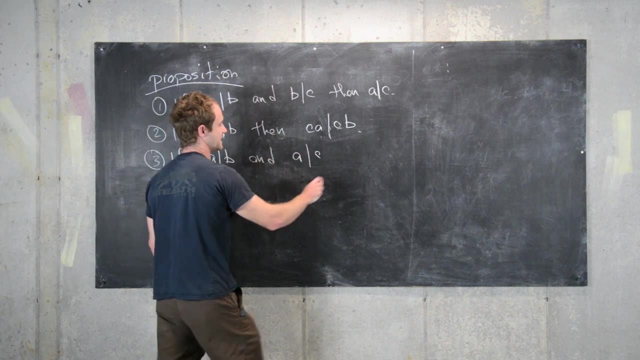 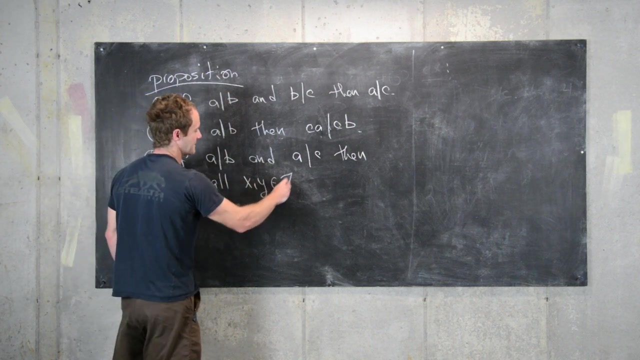 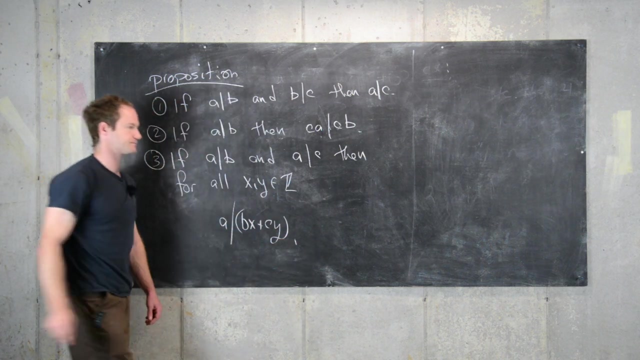 But it's easy to fill in those details. And then, lastly, is if A divides B and A divides C, then for all integers X and Y, we have A divides BX plus CY. Good, So I don't want to prove all of these. 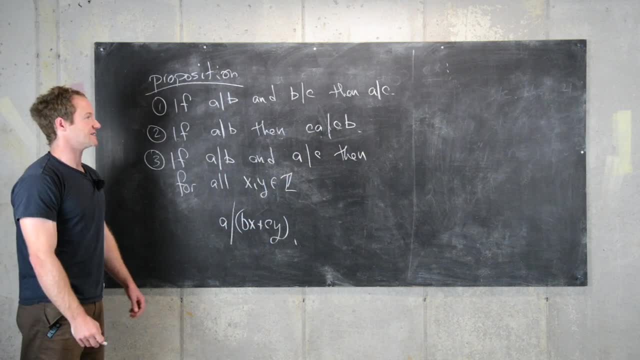 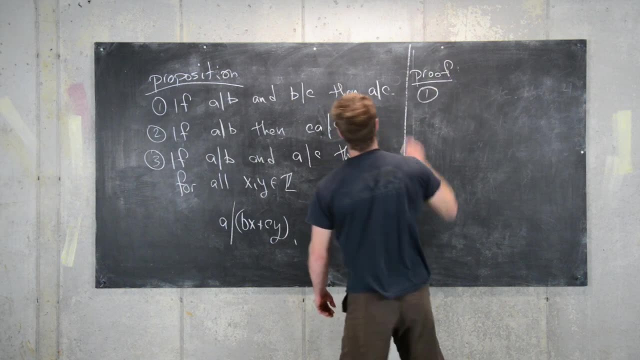 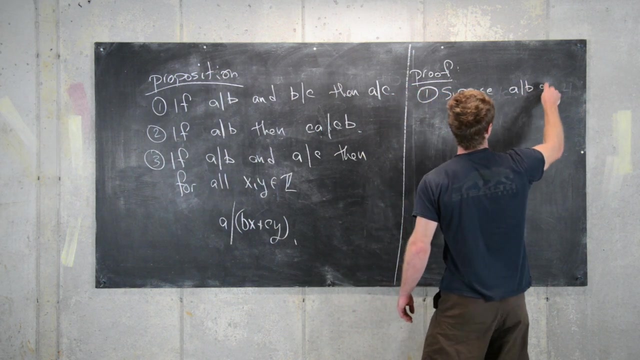 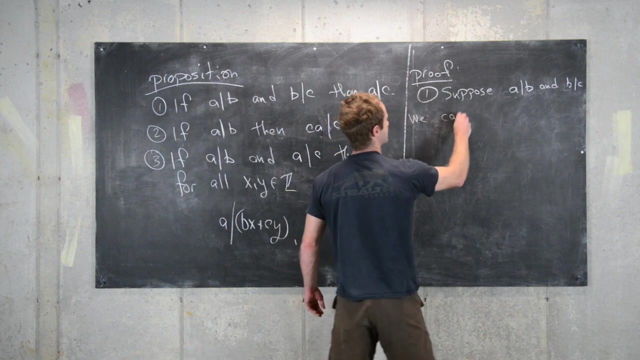 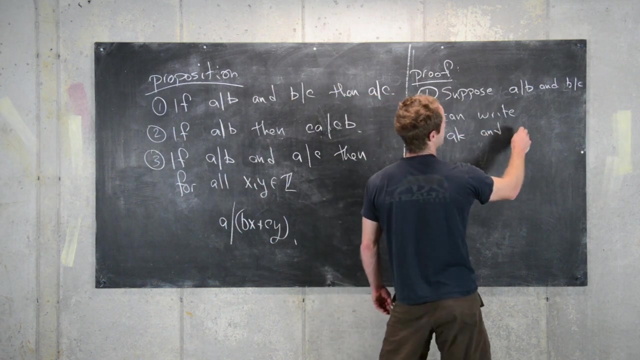 Maybe I'll prove number one and then the last two will be left as an exercise. So proof for number one. So let's suppose that A divides B and B divides C, So that means we can write: B equals A times K and C equals B times L. 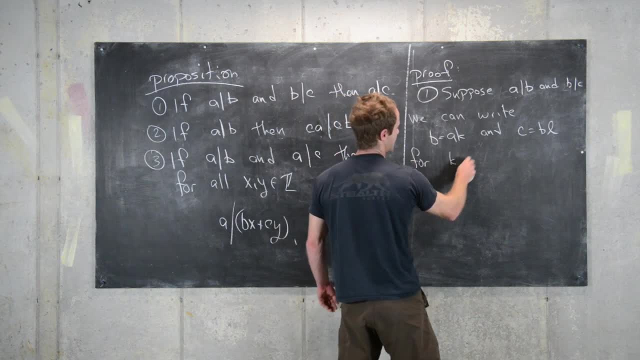 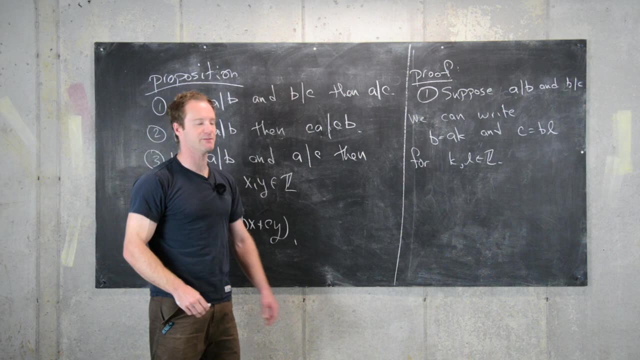 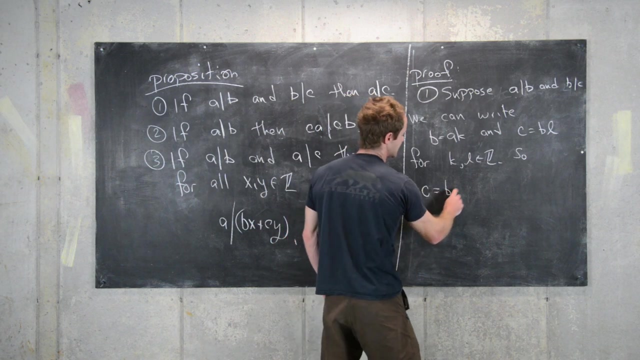 for K and L, some appropriate integer Good. The next thing we do is we match these two equations together And that will give us C equals B times L, which equals- we'll replace B with this, So that's A times K times L, Good. 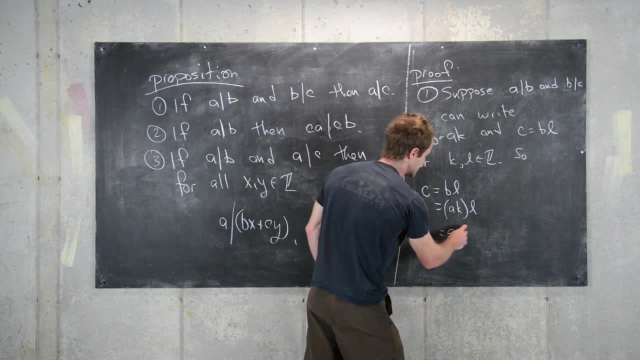 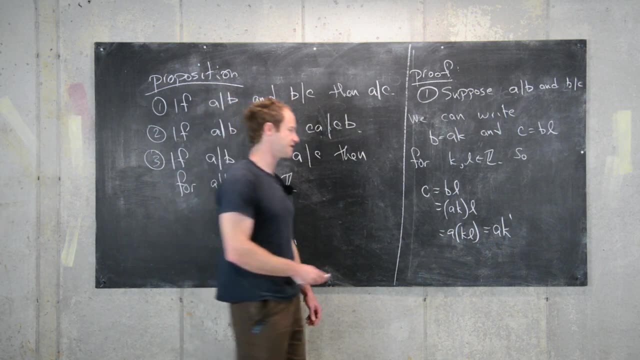 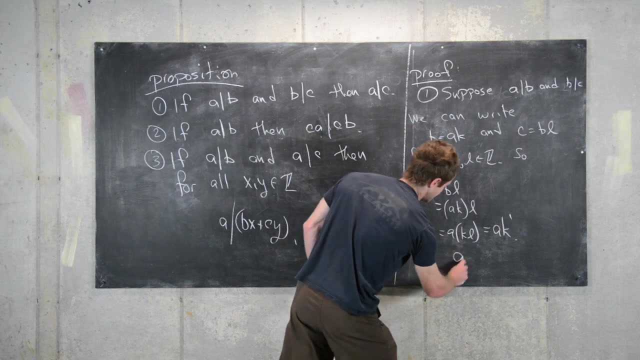 Now we can re-associate So that gives us A times K times L, which is A times K prime, And K prime is A times K prime, And K prime is A times K prime And K prime is another integer. Thus we have A divides C, as desired. 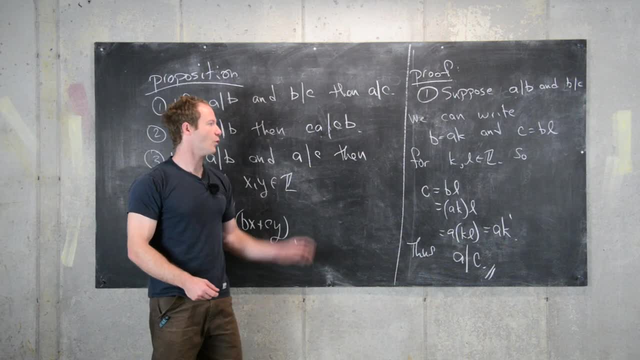 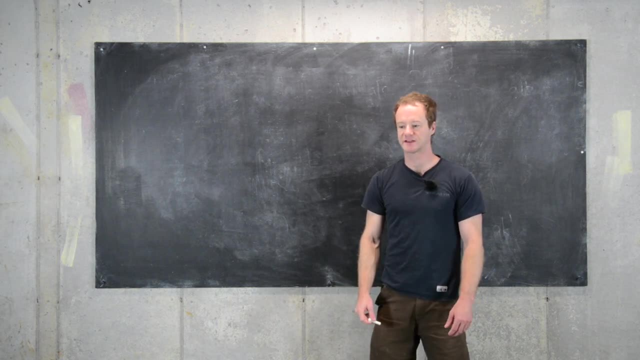 Okay, good. So before we end this video, I want to give one more result about divisibility. I'll clean up the board and then we'll do that, Okay, finally, I want to prove this last claim about divisibility, which is extremely useful. 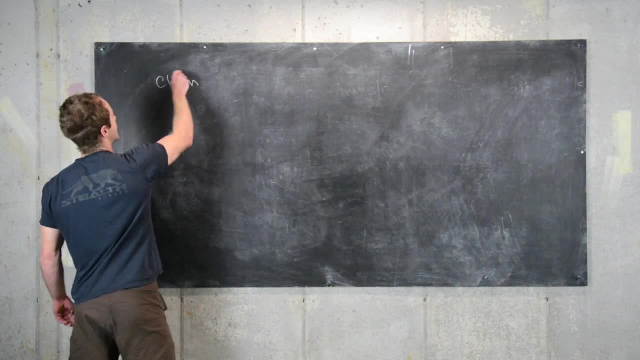 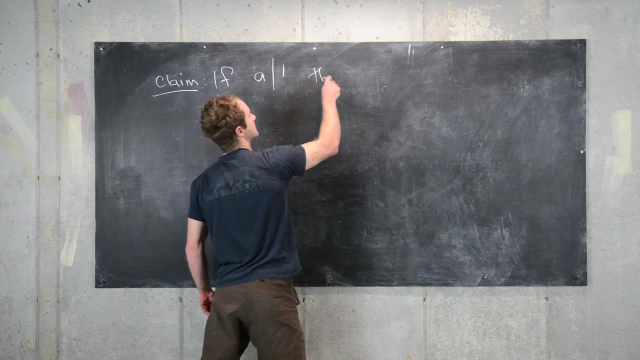 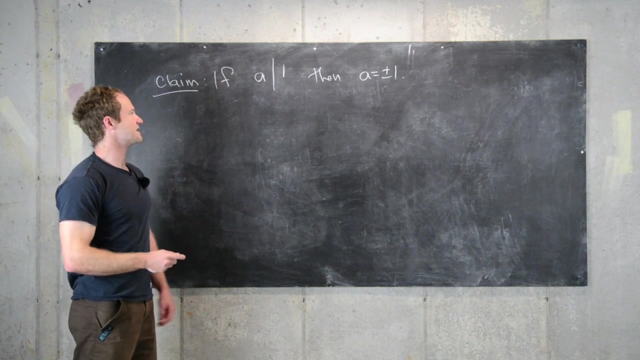 And that's the following. So claim: if A divides 1,, then A equals plus or minus 1.. Okay, good, So that makes sense, because if you have something that divides 1, it seems like it would have to be a fraction. 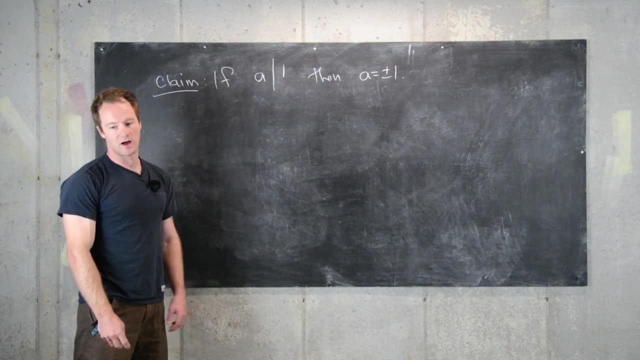 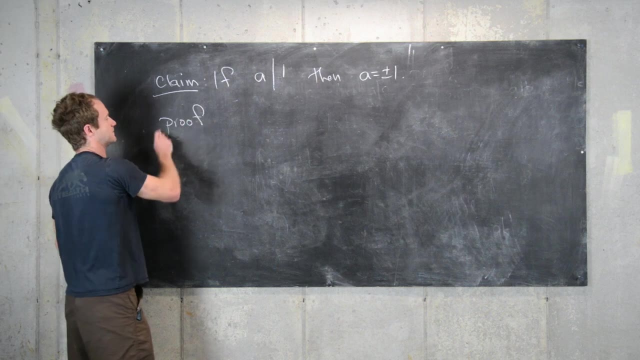 or it would have to be smaller than 1.. And that's exactly what we're getting at here, in terms of absolute value at least. Okay, great, So let's prove this. So let's suppose that A divides 1.. 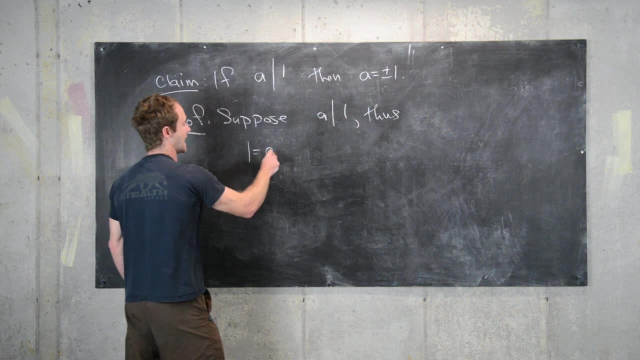 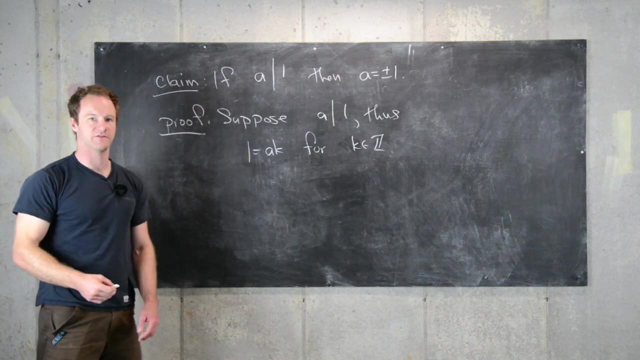 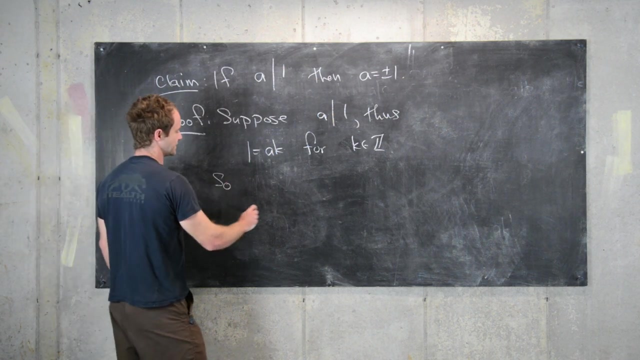 Thus we can write: 1 equals A times K, for some integer K, Okay, fantastic. And then what I want to do now is take the absolute value of this equation, So that'll give us 1 equals the absolute value of A times. 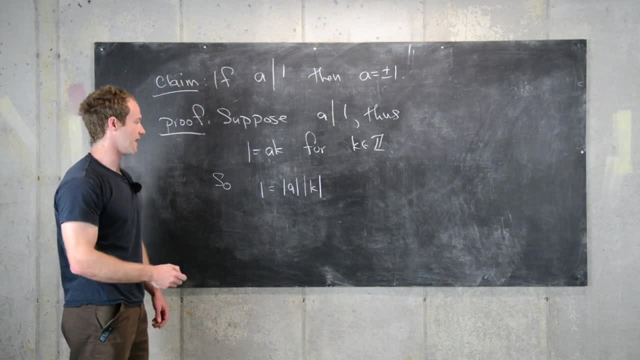 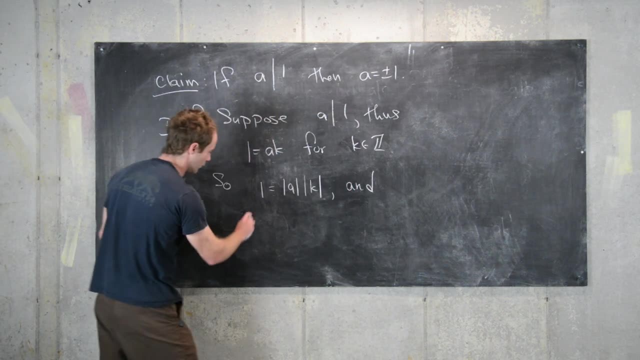 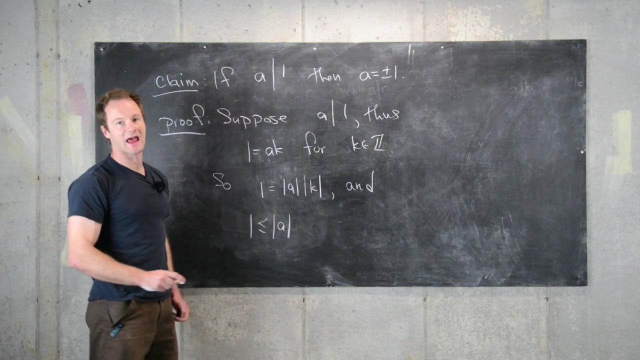 the absolute value of K. Okay, fantastic. And now that will build the following inequality: So 1 is less than or equal to the absolute value of A. So that's true because we're assuming that A is an integer. You know, the absolute value of any integer is bigger than or equal to 1.. 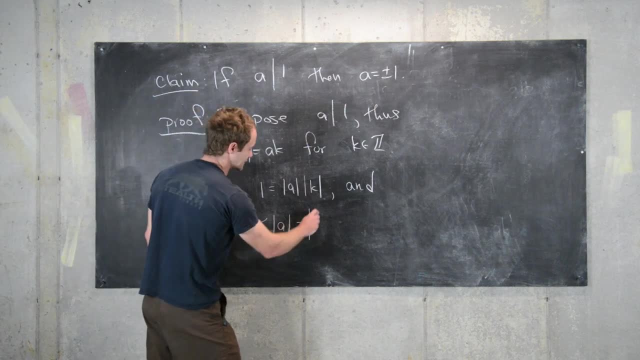 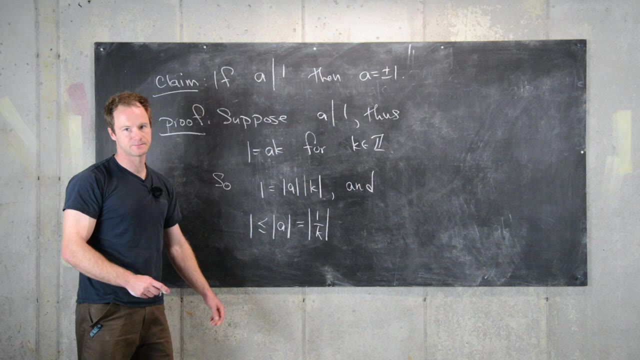 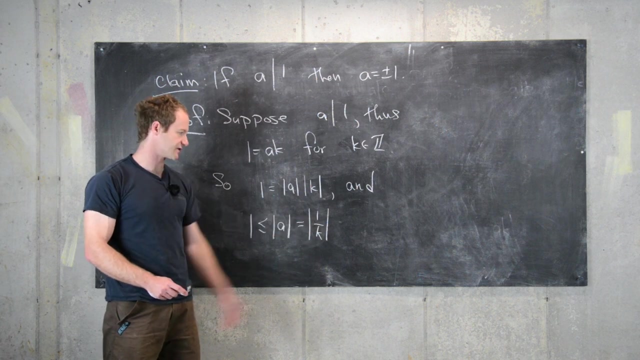 Good. And then that is equal to the absolute value of 1 over K. A good, just by this equation. And then, finally, since this is the reciprocal of an integer, but it's absolute value, this is the reciprocal of a natural number. 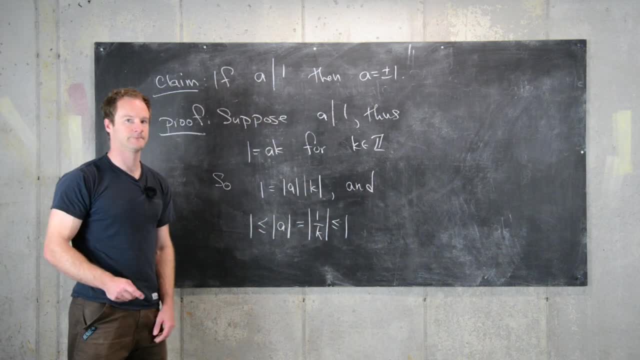 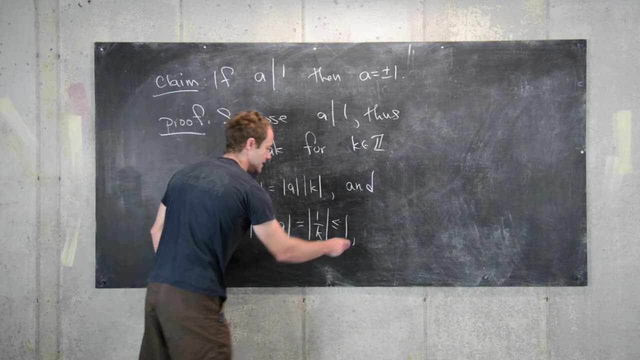 So that means this is less than or equal to 1.. So we end up with this sandwich: A is bigger than or equal to 1, and it's less than or equal to 1.. Thus the absolute value of A equals 1.. 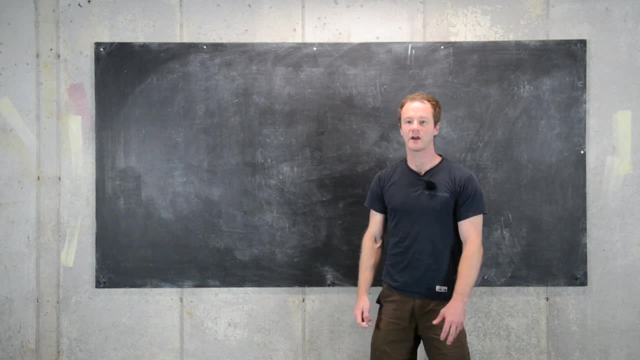 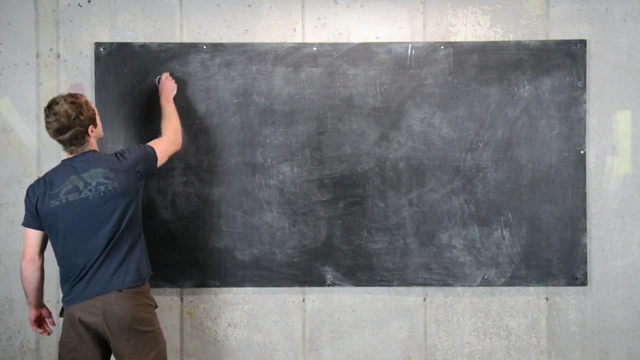 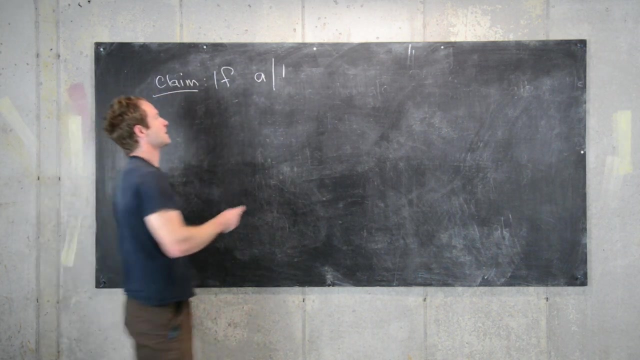 I'll clean up the board and then we'll do that. Okay, finally, I want to prove this last claim about divisibility, which is extremely useful, And that's the following: So claim: if A divides 1, then A equals plus or minus 1.. 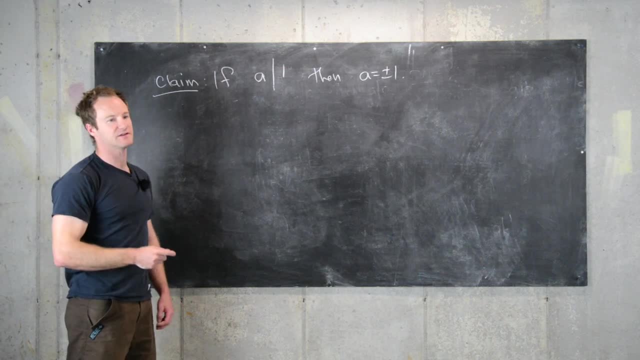 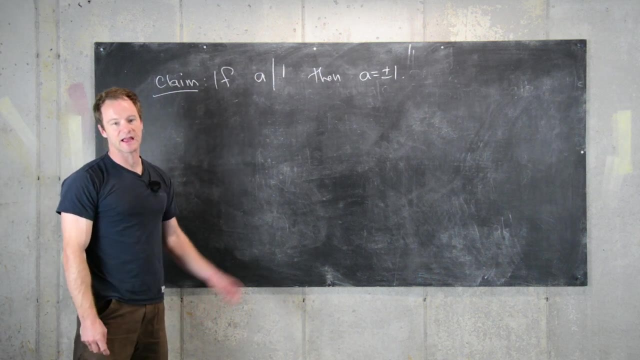 Okay, good. So that makes sense, because if you have something that divides 1, it seems like it would have to be a fraction, or it would have to be smaller than 1.. And that's exactly what we're getting at here, in terms of absolute value at least. 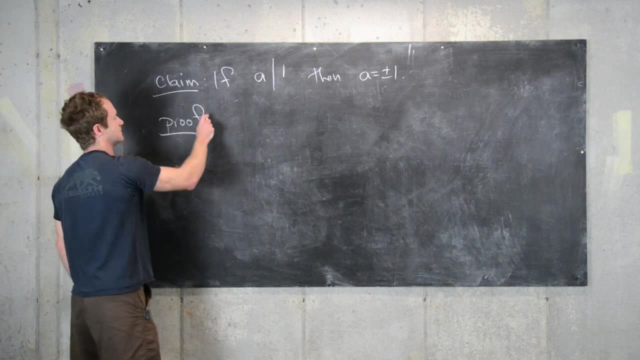 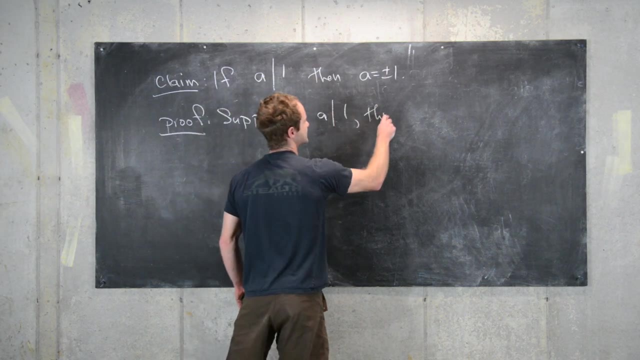 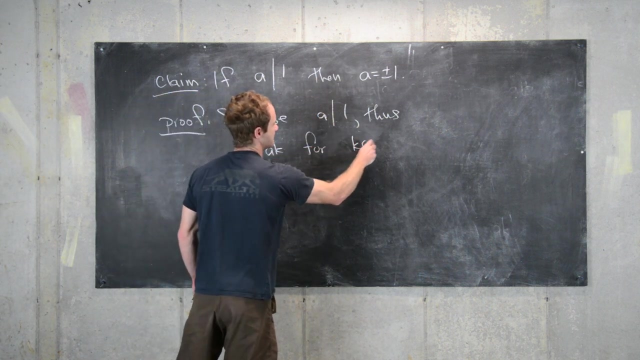 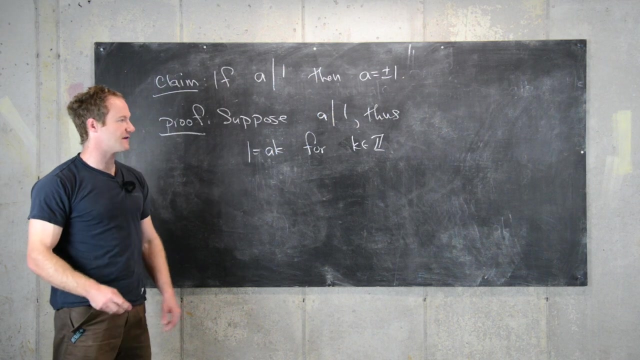 Okay, great. So let's prove this. So let's suppose that A divides 1.. Thus we can write: 1 equals A times K for some integer K, Okay, fantastic. And then what I want to do now is take the absolute value of this equation. 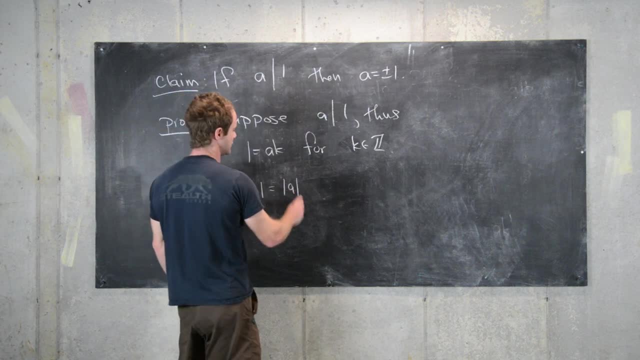 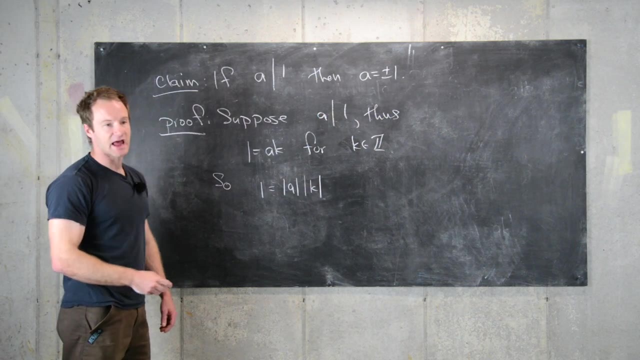 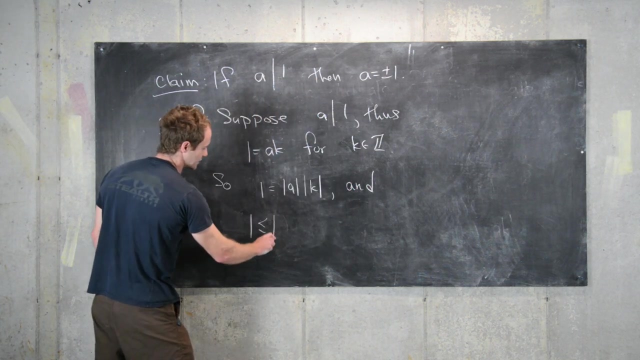 So that'll give us: 1 equals the absolute value of A times. So that'll give us: 1 equals the absolute value of A times the absolute value of K. Okay, fantastic. And now that will build the following inequality: So 1 is less than or equal to the absolute value of A. 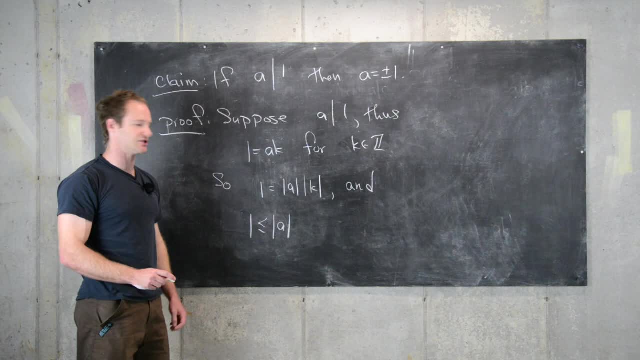 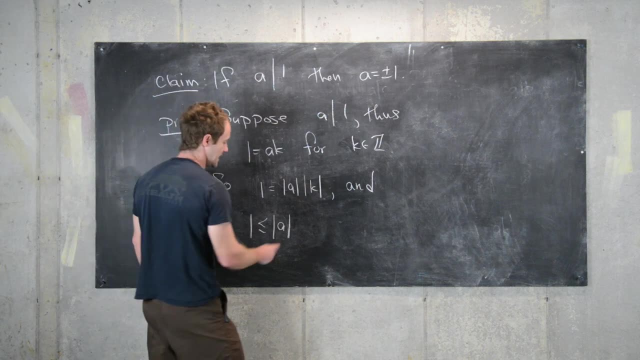 So that's true, because we're assuming that A is an integer. You know, the absolute value of any integer is bigger than, or equal to, 1.. Good, And then that is equal to the absolute value of 1 over K. Okay, 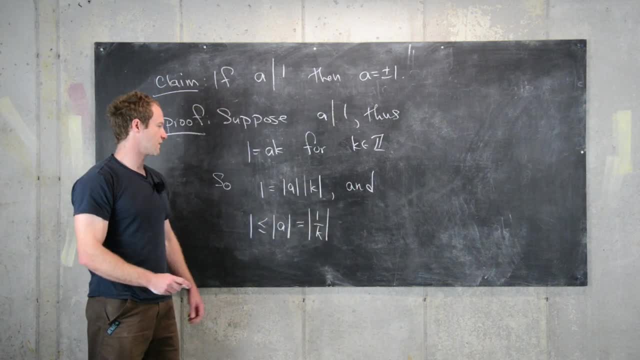 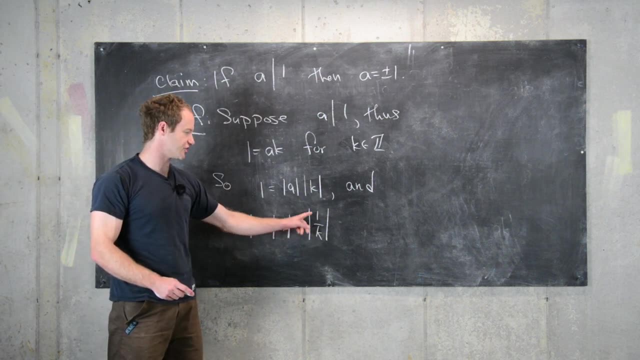 Good, Just by this equation. And then, finally, since this is the reciprocal of an integer but its absolute value, this is the reciprocal of a natural number. so that means this is less than or equal to 1.. So we end up with this sandwich. 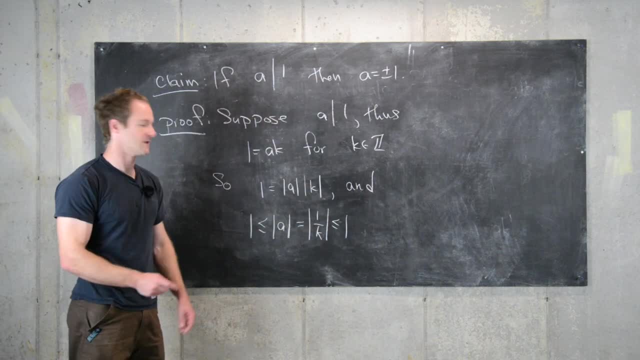 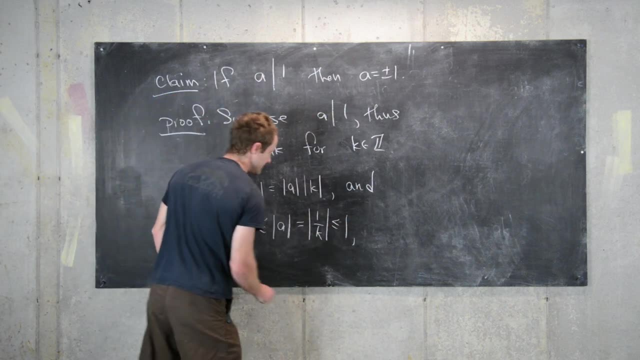 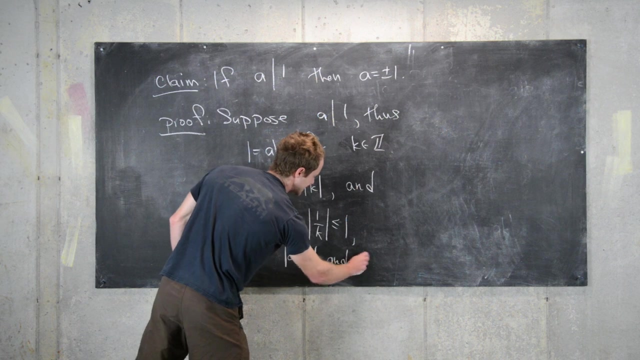 A is bigger than or equal to 1, and it's less than or equal to 1.. Thus, the absolute value of A equals 1.. So let's say that this is the absolute value of A. Okay, The absolute value of A equals 1, and that means that A equals plus or minus 1..